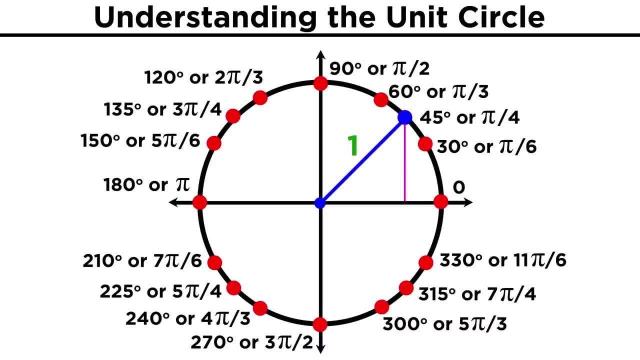 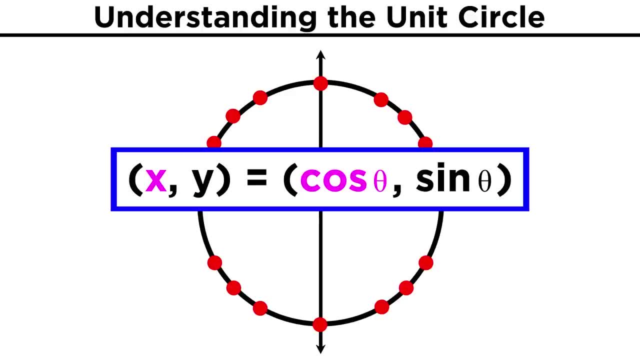 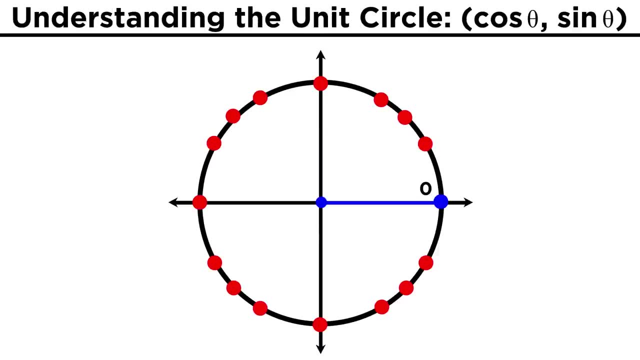 two legs are each some value less than one, depending on the angle. What we must understand is that every point on this unit circle has an X coordinate equal to cosine theta And a Y coordinate equal to sine theta. Take zero as an example. 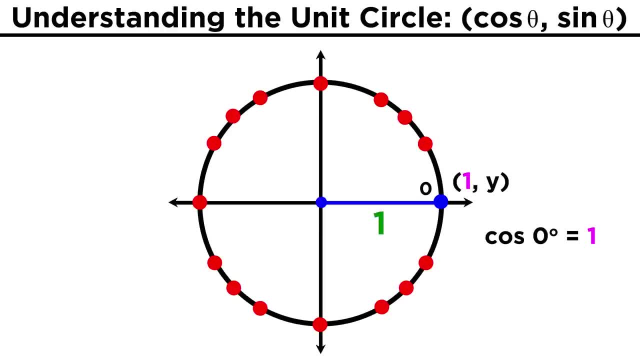 There is no triangle, but since the radius of the circle is one, we know that the cosine of zero must be one because the X coordinate of this point is one. Likewise, we know that the sine of zero must be zero because the Y coordinate of this. 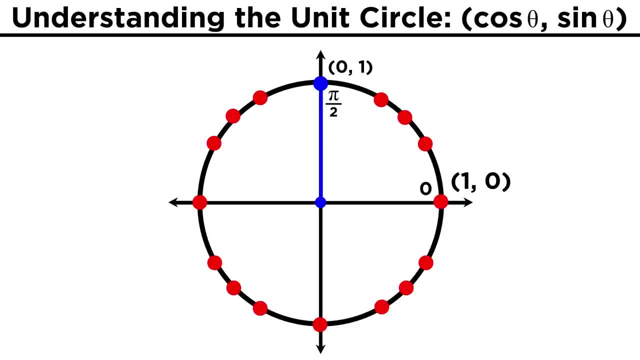 point is zero, It will be just as easy to figure out the values For half pi as this point has the coordinates zero, one. So the cosine of half pi must be zero, while the sine of half pi must be one. At pi, we get negative one and zero. and at three halves pi we get zero and negative one. 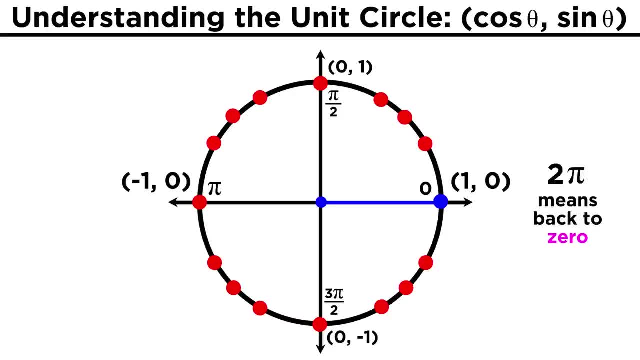 Once we make it to two pi, we are back where we started and the cycle continues. Now what's important to see? What's important to see is that the cosine and sine of any angle other than these must be somewhere in between negative one and one. 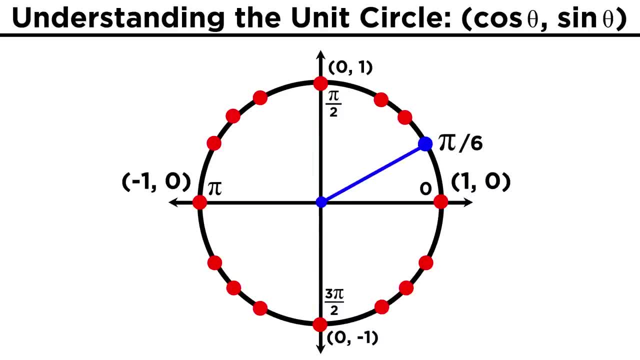 Let's take pi over six, for example. In the last clip we evaluated the trig functions for these two special triangles, so if you missed that, go check it out now. Otherwise, just take my word for it that the sine of pi over six radians or thirty degrees, 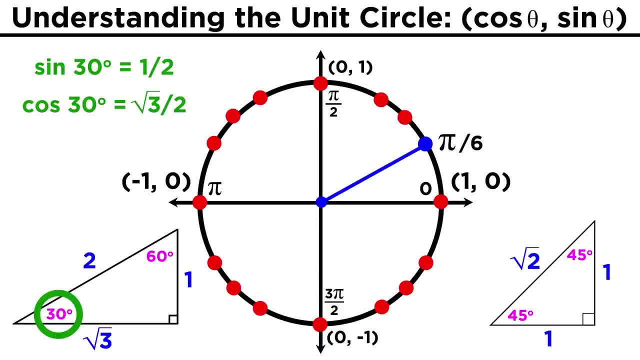 is one half And the cosine is root three over six. That means that the coordinates of this point are root three over two, one half. For quarter pi we have this other special triangle and both the sine and cosine of forty-five are root two over two. 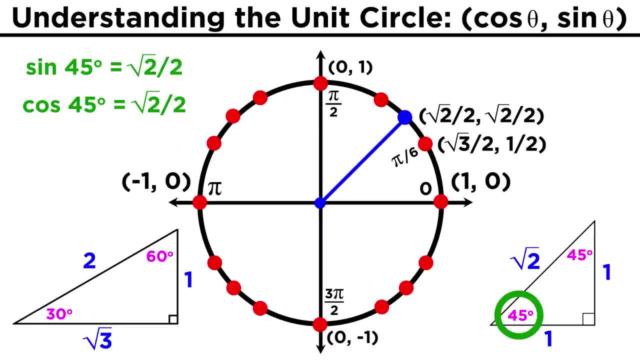 So these are the coordinates of this point. For two, pi over six or pi over three, we have the same values as for pi over six, but reversed It's the same triangle, just looking at the other angle. That means that these are the coordinates of this point. 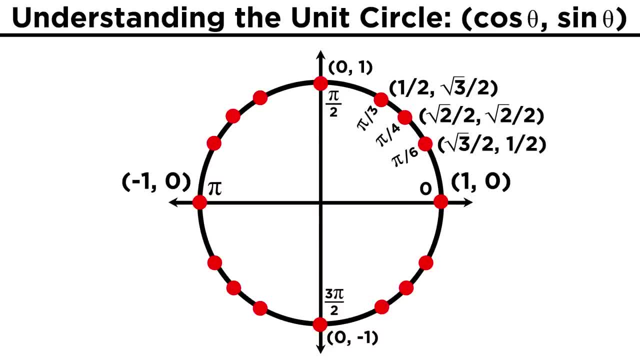 And that wraps up the first quadrant. Now here's the thing that makes this so easy to remember. We see some fractions and some roots which may seem unrelated. Just for the sake of creating a pattern, let's replace zero with root zero over two, since 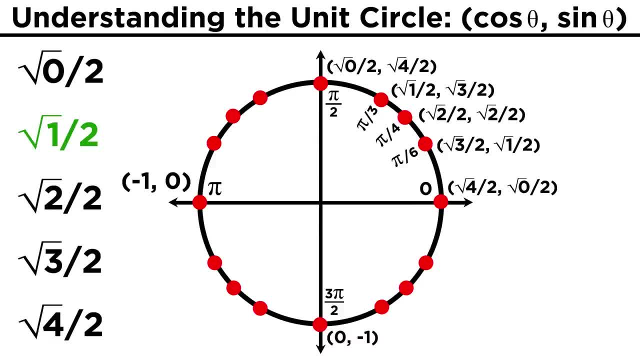 root zero is zero. Let's change one half into root one over two, Since root one is one. Then we have root two over two, root three over two, and let's change one into root four over two, since root four is two and two over two is one. 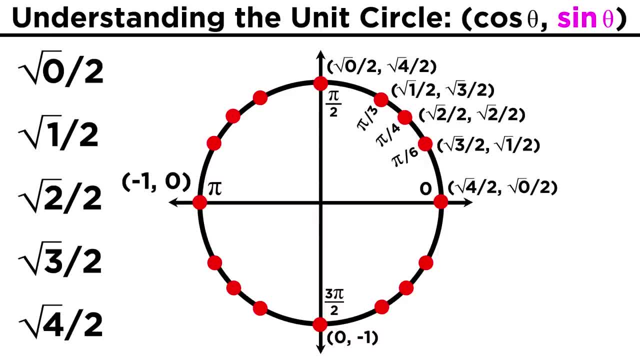 Now, if we look at the sine values for these angles, which correspond to the Y coordinates of the points, we can start at the X axis, where the Y value is root zero over two. we climb up to root one over two, then root two over two. 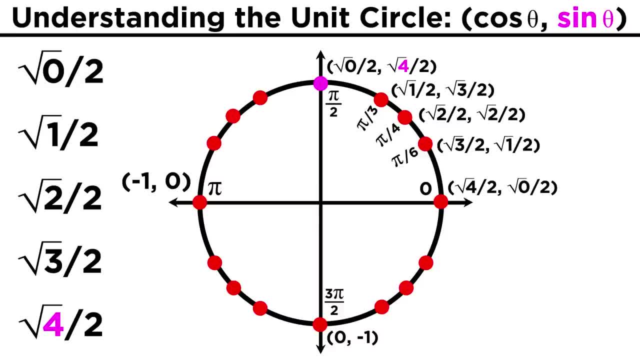 Then root three over two, then root four over two. We could do the same thing with the X values, which correspond to cosine values for these angles, starting with the Y axis and then moving to the right in the positive direction. Again we hit the same values. 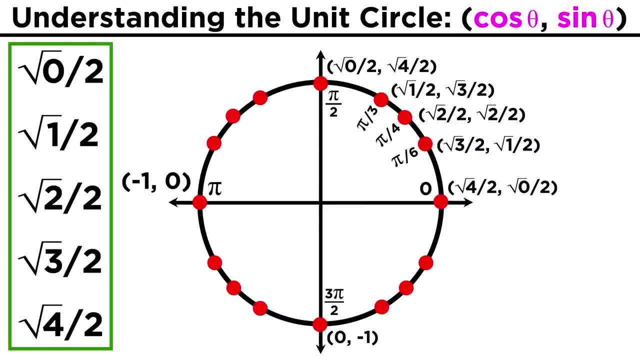 So all we have to do is remember this one numerical sequence and that the coordinates of each point take the form of zero, So we can start at the Y axis and then move to the right in the positive direction. Again, we hit the same values. 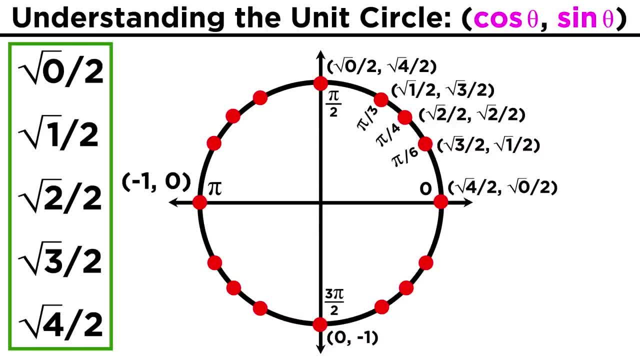 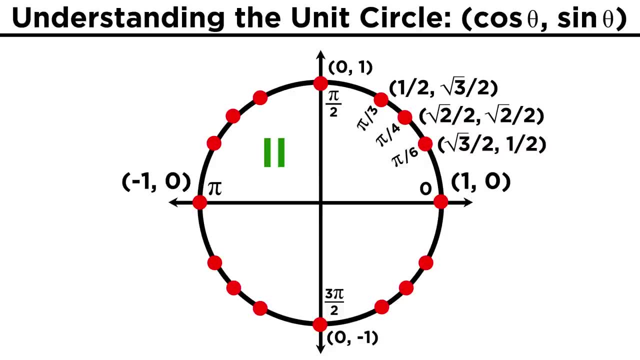 So all we have to do is remember this one numerical sequence and that the points take the form of cosine, theta, sine theta, and we will never forget any of these values. Let's return these values to their simplified forms and then extend things into quadrant. 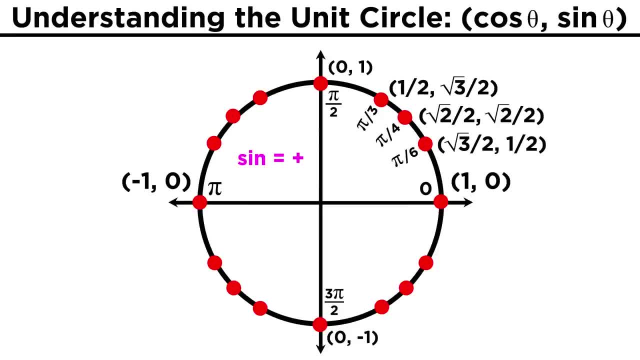 two, We can see that sine values or Y coordinates will remain positive, as these points are above the X axis. Five-sixths pi will have a sine of one-half, just like one-sixth pi. Three-quarters pi will have one-thirty, though reason-based Eigenvalue. 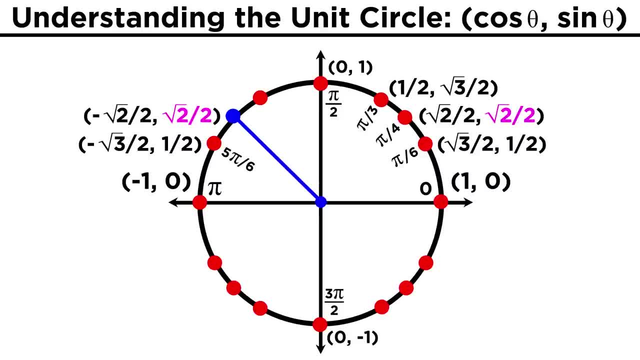 quarters pi will have a sine of root two over two, just like quarter pi. Two thirds pi and one third pi each have a sine of root three over two. Now for the cosine values. it's the same thing, except that they are now negative. 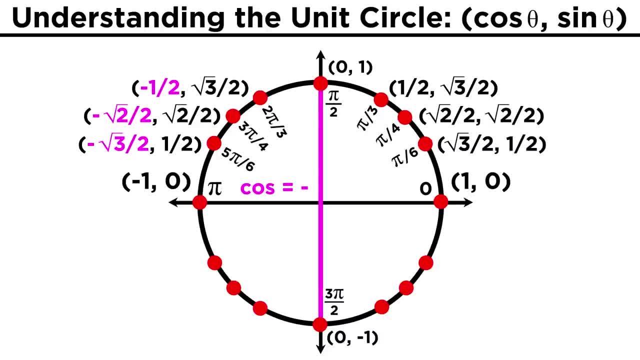 as they are to the left of the Y axis. Going into the third quadrant, both sine and cosine become negative, as X and Y are both negative, but it's still all the same numbers. And into the fourth quadrant, cosines return to being positive while sines remain negative. 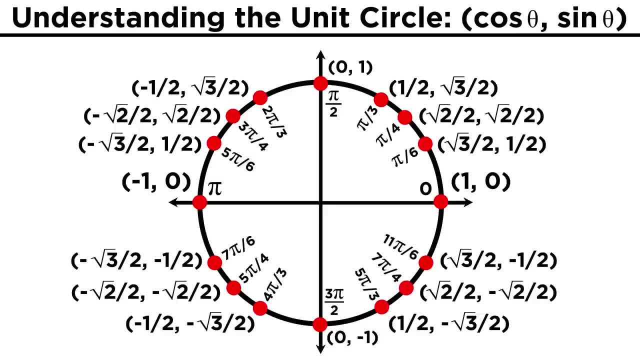 Knowing this, we could take any of these angles and immediately know the sine and cosine simply by visualizing the unit circle. Take four thirds pi, for example, To get the sine of this angle, we simply locate the angle which can also be thought of as this reference angle or one third pi. but 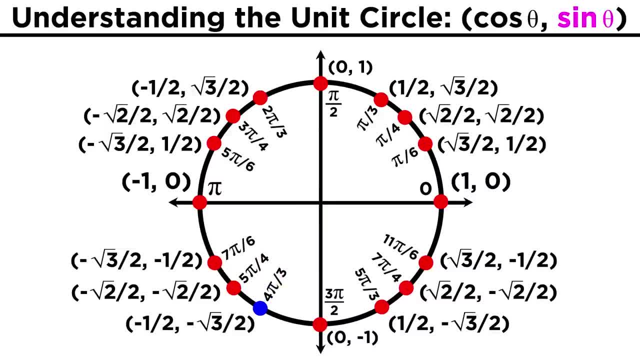 in quadrant three. Then we recall that sine corresponds to the Y coordinate of this point and we just move downwards until we get there Zero, negative one, half. negative root two over two, negative root three over two To get the cosine value. we just remember that cosine corresponds to the sine of the 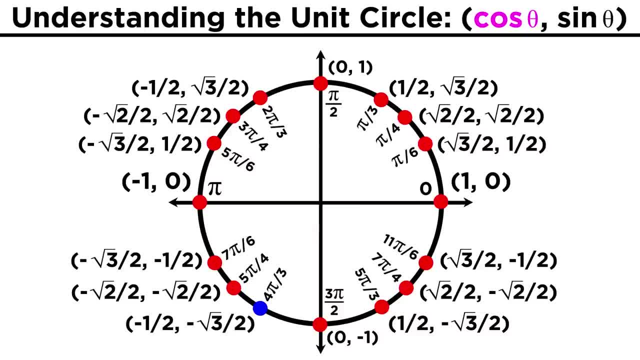 unit circle To get the cosine value. we just remember that sine corresponds to the X coordinate of the point Zero negative one half. We aren't calculating anything, we just have to memorize the locations of the angles, this one numerical sequence, and what the coordinates of the points represent. 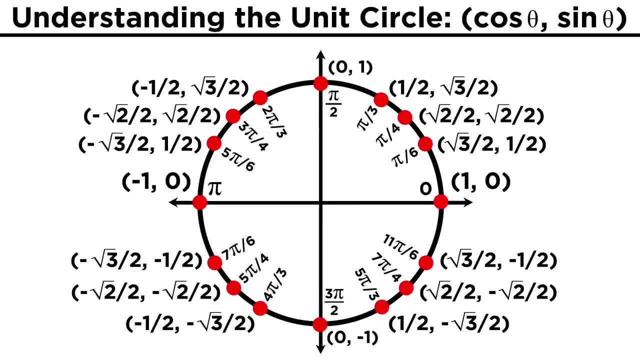 Once this is ingrained in you, you'll never forget it. so just stare at this until it makes sense. When you have it, it becomes trivial to evaluate trig functions for any common angle. Take something like the tangent of fourteen pi over three. 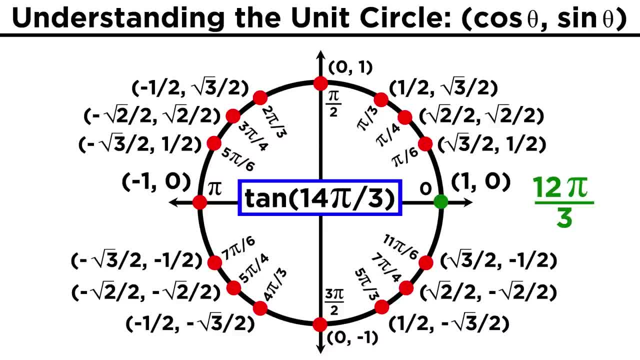 Twelve thirds pi is the same as four pi and that's twice all the way around. so we can subtract that from the angle to get two thirds pi. That gets us right here Now. tangent is sine over cosine, so let's take the Y value of this point and divide. 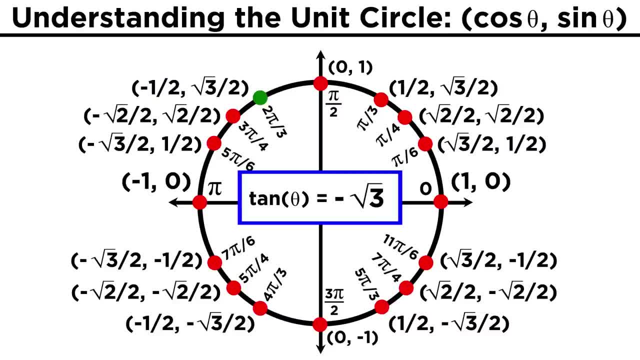 by the X value of this point, And that gives us negative root three. What about the cosecant? It's a constant. What about the cosine secant of negative 17 fourths pi? This time we are going in the negative direction.